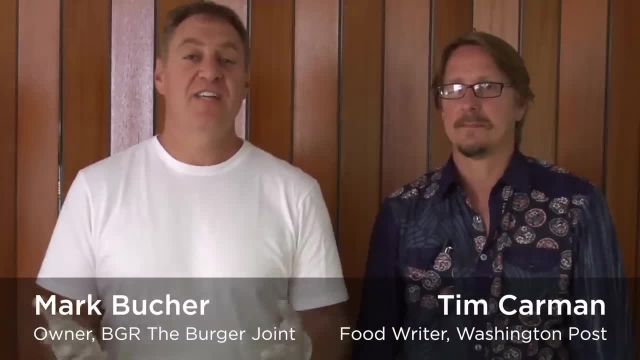 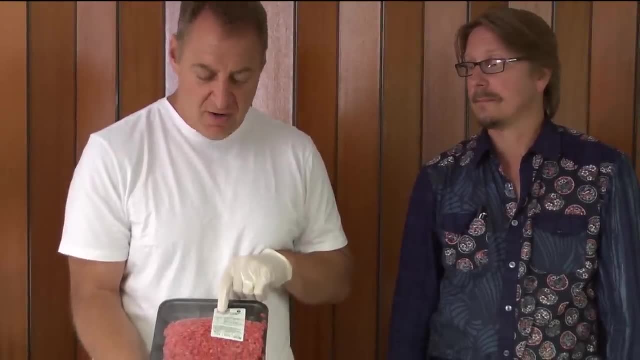 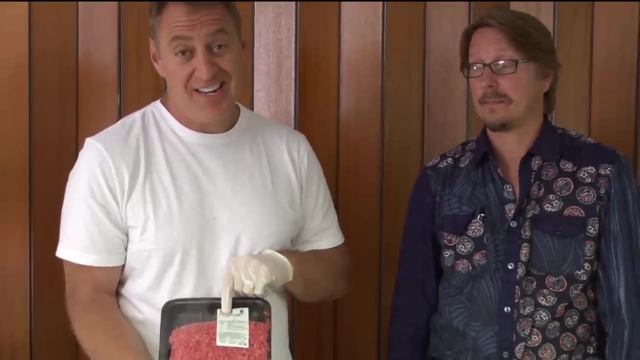 Today we're going to learn how to make burger patties at home the right way, because you've been making it wrong all these years. Lean ground beef does not make a good burger. You want at least 20% fat, If not more. If not more, At least 20% fat I would try to get. 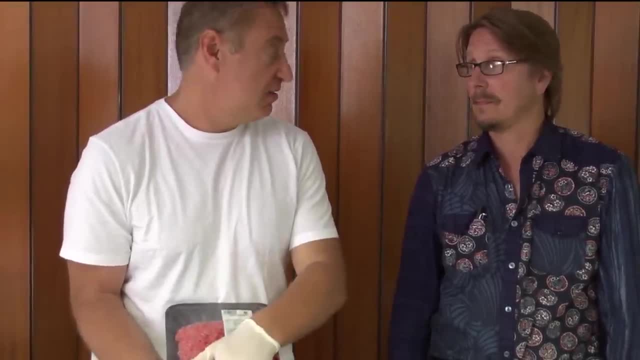 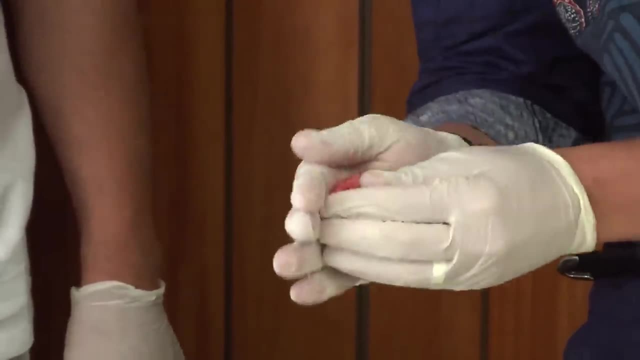 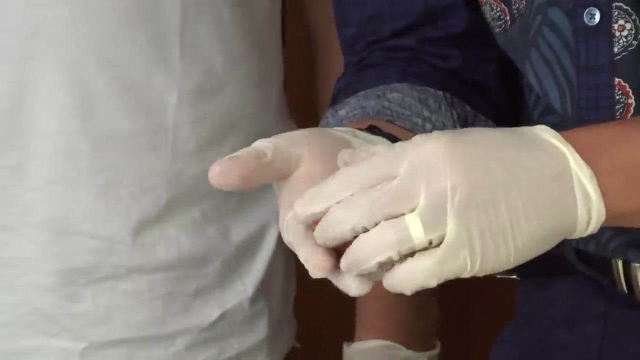 25% fat And I would look for ground chuck. When I make a patty, I don't want to form it too much. I want to keep it loosely formed, because when you cook something that's been pressed together too much, it's going to turn it into like my father used to call them. 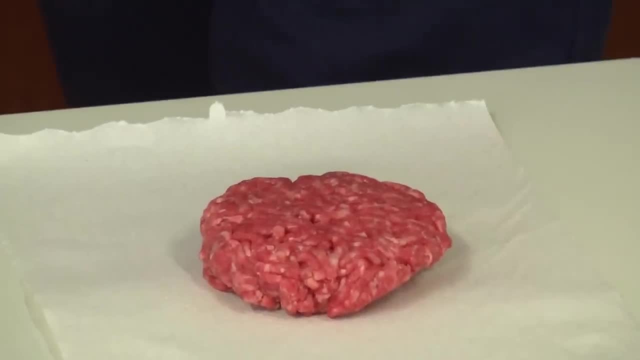 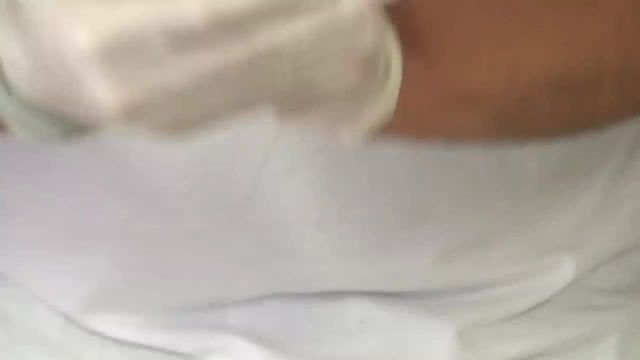 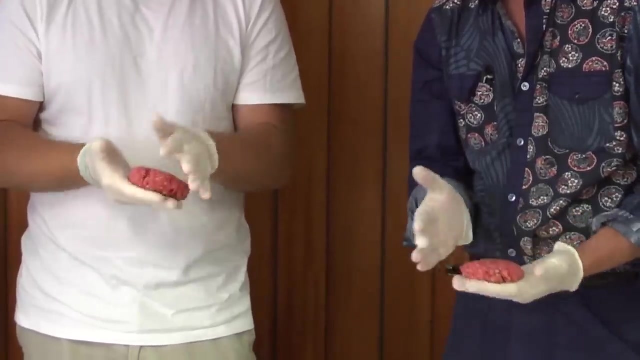 hockey pucks. You know a lot of manly men will, you know, really get in there and really make this? you know I got this, I'm really making it something, And I think that's wrong. You got to be gentle, Gentle. 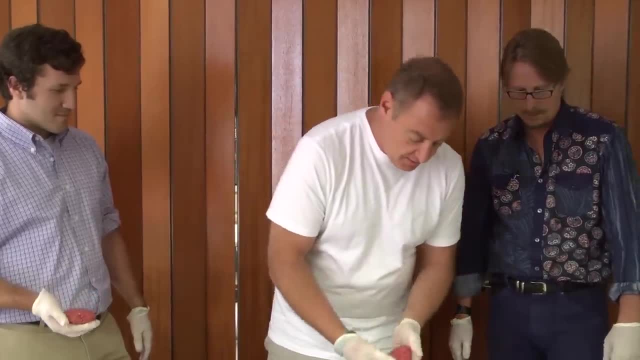 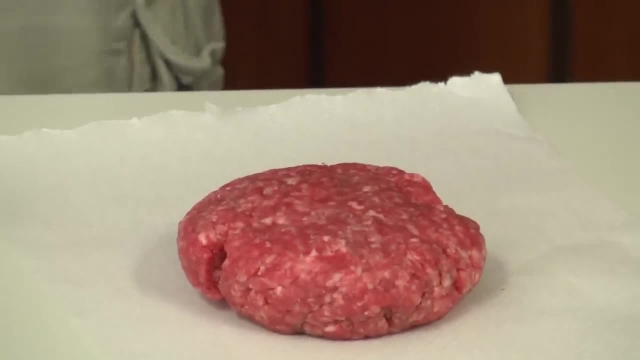 Well, the other trick here is: once you've got your burger done, you know you set it down and you think you're all good to go. One of the tricks that I've learned is the old thumbprint in the center. Have you ever seen that before? 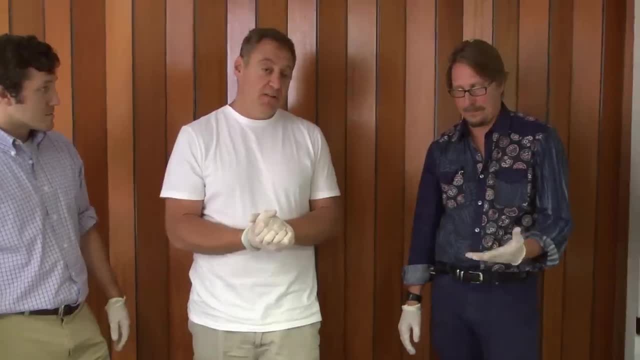 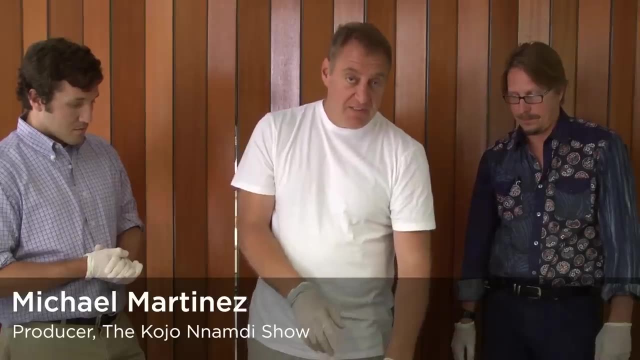 So that A keeps it from balling up. You know, when you take fresh beef and you put it on or you cook it, it will all tighten and it will ball up like a golf ball. So this allows it to cook evenly in the center and it will keep it flat. 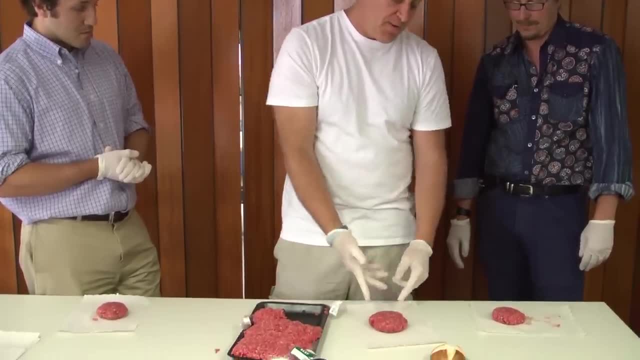 The other trick I do is I refrigerate it before I put it on the grill. I'll put it in the refrigerator for about 15 or 20 minutes, let it cool back down again before I put it on the grill. I think people under season. 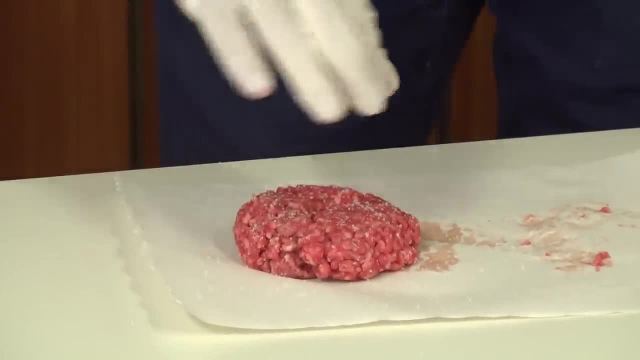 I think people are always afraid of salt and pepper when they cook and don't forget a fair amount of it actually falls off. I don't put salt and pepper inside the meat. I won't put it in a bowl and put salt and pepper and mix it up. I also won't put salt and pepper on a burger a long time before I cook it. I'll put it on right before I cook it, Because if you put salt on too soon, it will pull all the moisture out of the burger And then liberally season with pepper. 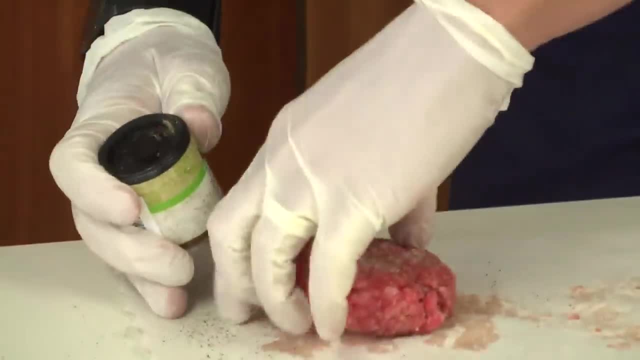 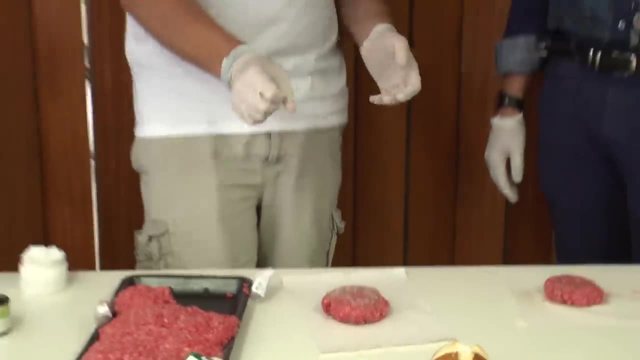 I mean personally. I love a lot of pepper on a burger. When I put it on the grill, I will put it seasoning side down, then I'll season the other side on the grill. My other rule on the grill is: put it down, don't touch it.